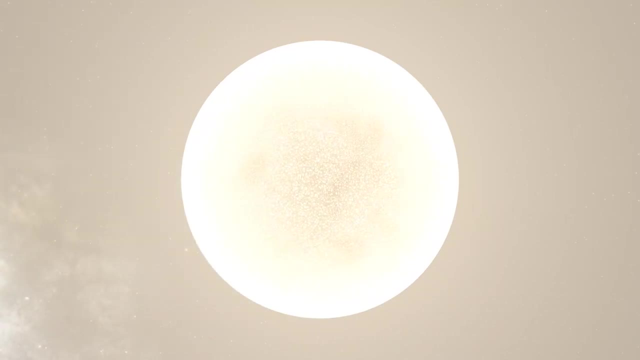 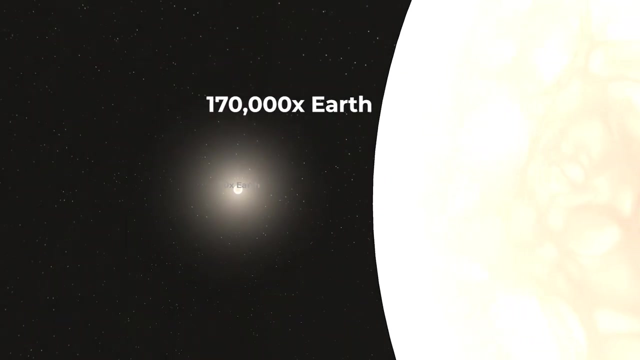 Stars are the largest singular structures in our universe, ranging from 10 times the size of the Earth to a staggering 170,000 times. That's right. our Sun is small compared to most stars out there, which is also the reason why astronomers call it. 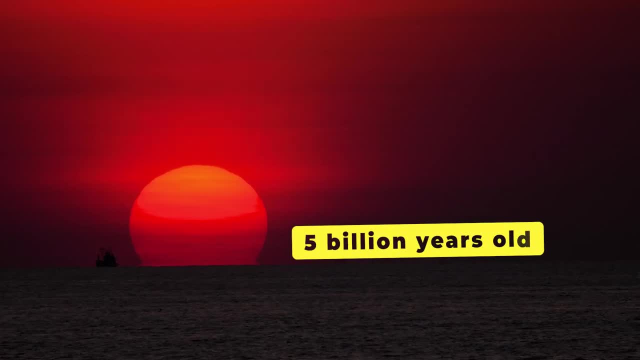 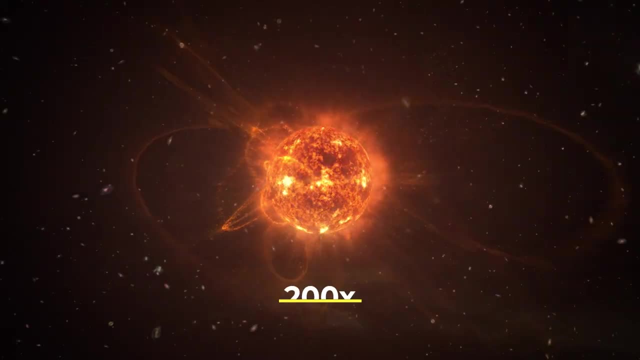 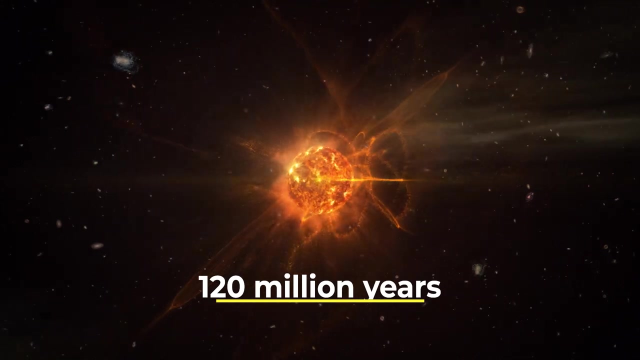 a yellow dwarf. Our Sun is roughly 5 billion years old, and we expect it to live for another 5 billion years, after which it grows over 200 times in size to become a red giant. It will only live on for a short 120,000,000 years in this stage before it sheds its 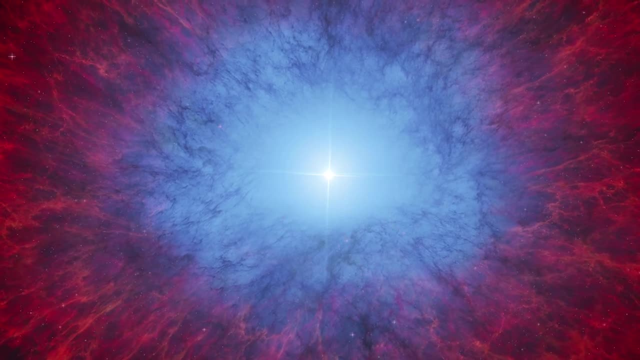 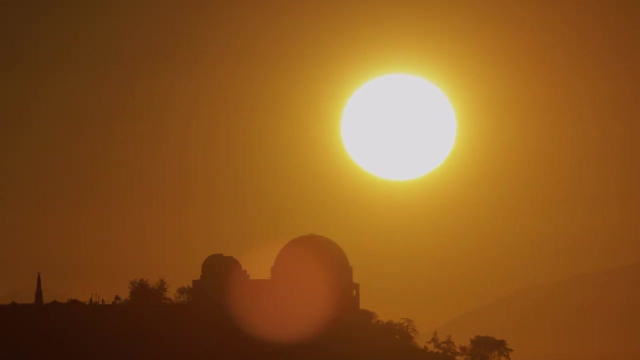 outer layers and becomes a white dwarf inside of a planetary nebula. Now you may wonder how we know these things and how things are different for other stars. Also, what about supernovae in black holes? Yes, we'll get there soon, But first what are our supernovae that are so different from other stars? Let's find out and we'll share with you the key answers. Also, what are our supernovae that are so different from other stars? Let's see and we'll share with you the key answers. First, what are our supernovae that are so different from other stars? 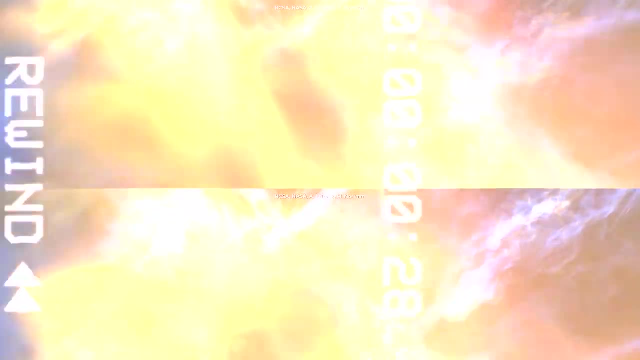 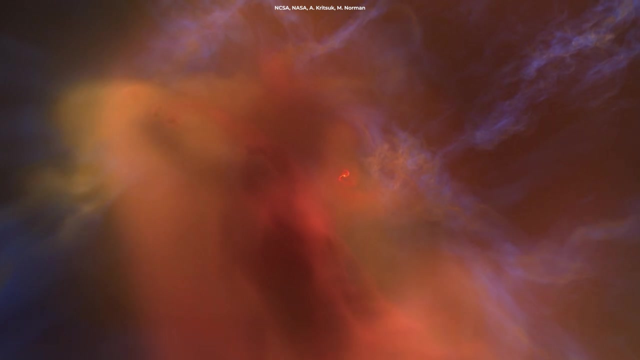 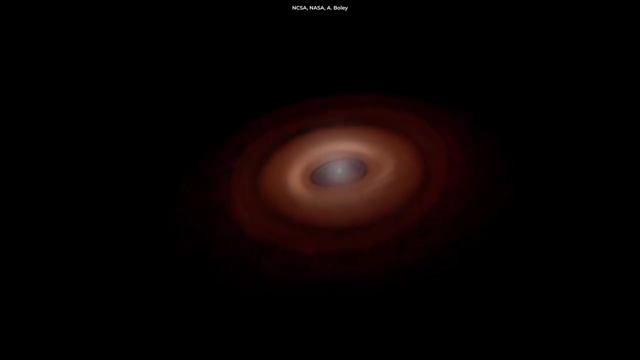 have to discuss the way that stars are born. This happens inside of a molecular cloud, which is basically a large collection of space gas that slowly but surely starts coming together due to the gravity of each individual dust grain Over the course of billions of years. 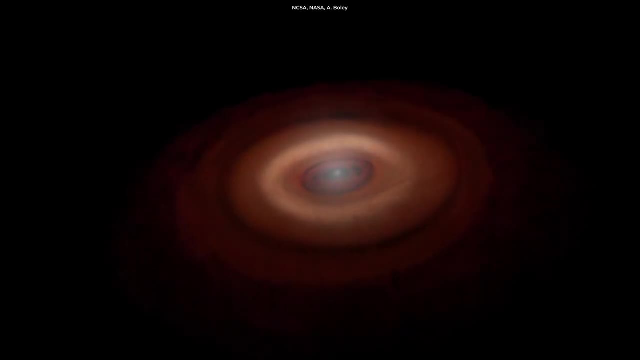 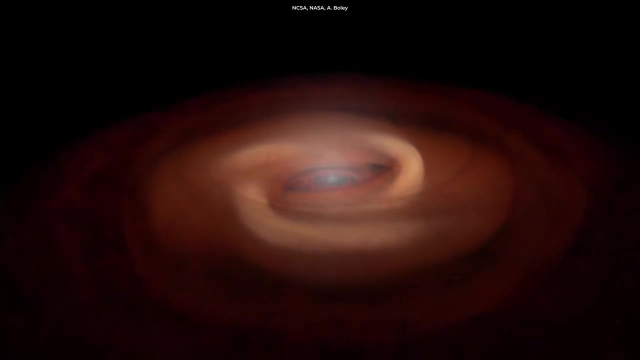 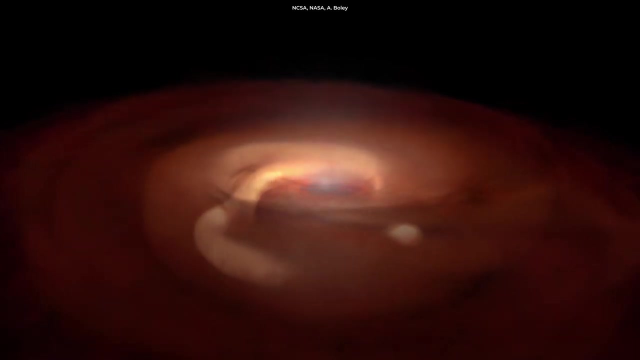 this cloud contracts so much that it starts to form a clump, somewhat even say a ball. This is where the entire future of the star is decided, because the weight of this clump will decide the size, lifetime and even the way it dies. Everything comes down to its initial mass. 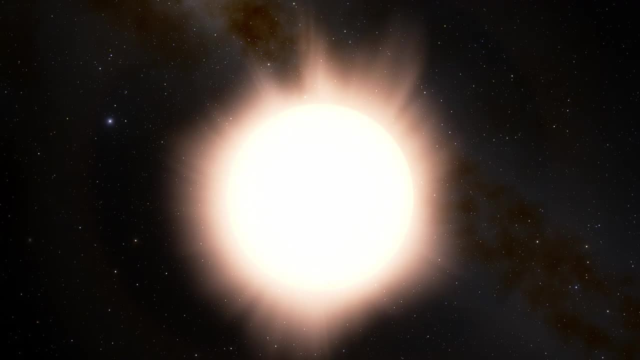 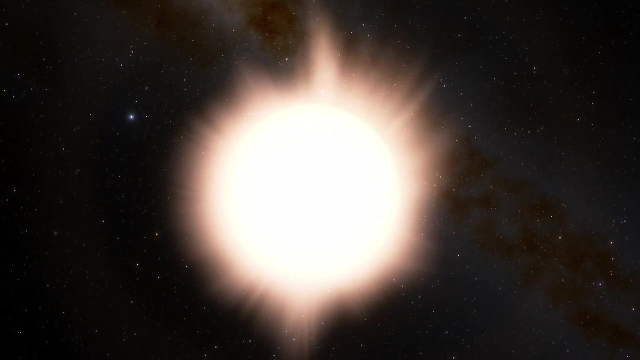 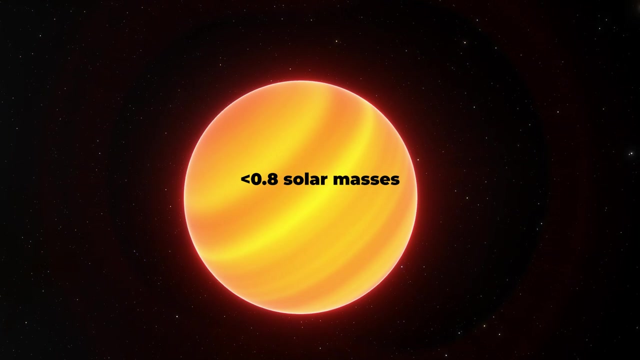 and typically this is expressed in solar masses, because it's easier to remember that the sun weighs one solar mass rather than 4.3 billion billion billion billion pounds. So, starting with the smallest first, a cloud that weighs less than 0.8 billion billion, billion, billion, billion billion. 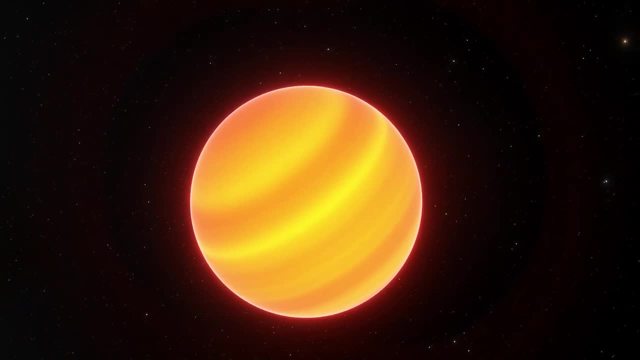 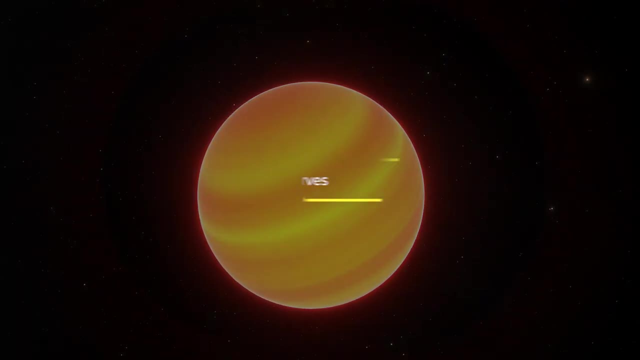 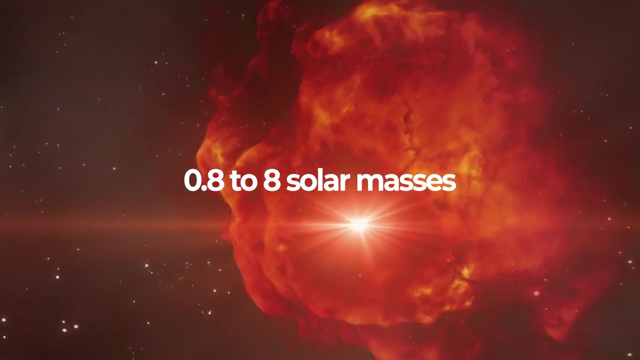 solar masses will not become a star. It's not heavy enough for the core to ignite, and thus it remains cold and dark. We call these objects brown dwarfs or failed stars. A cloud that weighs between 0.8 and 8 solar masses will become what is known as a low-mass star. These stars look and. 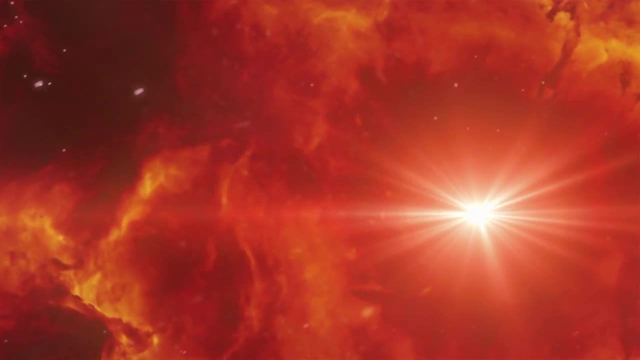 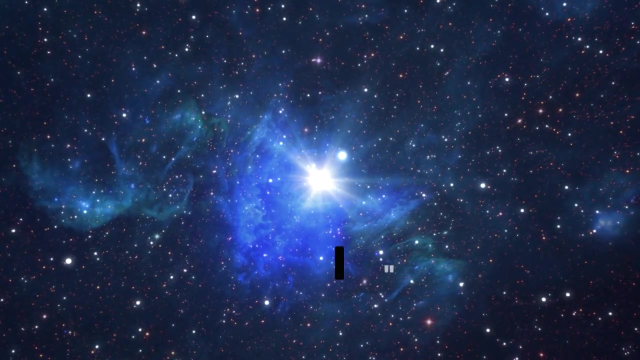 behave very much like our sun and live in a similar manner. The main difference is that the heavier stars burn much faster than the stars that are heavier than the stars that are heavier than the sun. Just like the old saying goes: burn bright, die young. And we're not kidding when we say young. 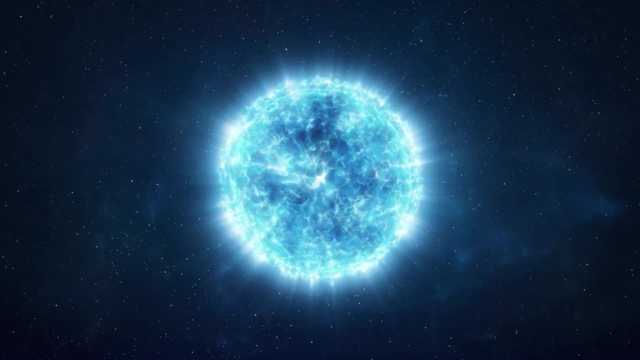 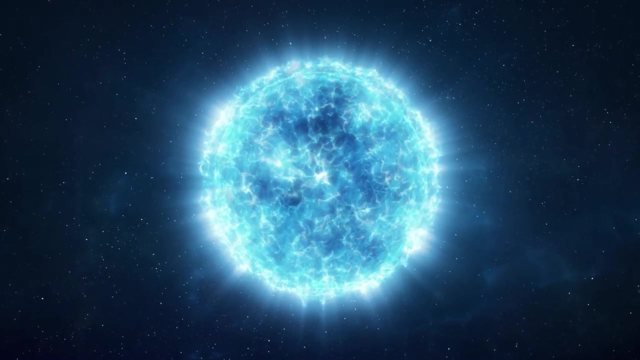 as an 8 solar mass star only lives for about 50 million years, a staggering 200 times shorter than our own sun. This is because the higher pressures in the star burn more hydrogen, thus depleting its resources at a faster pace. Then, once there's no more hydrogen to burn, the star expands into a red giant and starts burning helium in its core. This process doesn't create as much energy as burning hydrogen does and also uses up the available fuel much faster. Once this happens, the core starts contracting. 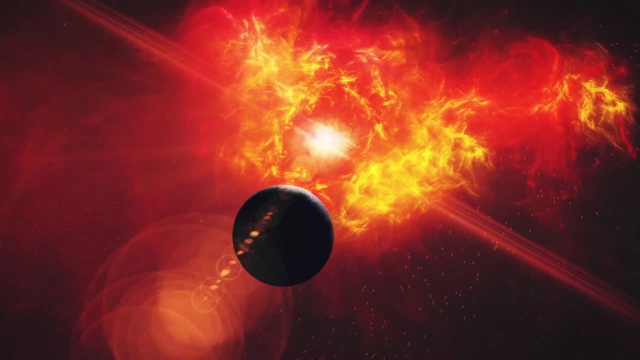 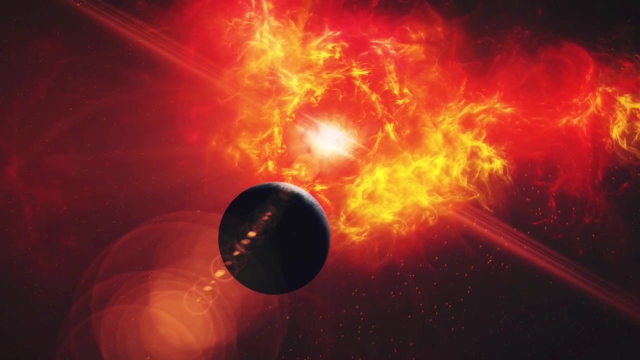 under its own gravity, dragging along bits of unburnt helium and igniting it in small flashes. These flashes aren't enough to stop the core from contracting, but do blow away more and more of the star's outer layer. Eventually, all of it is blown away into 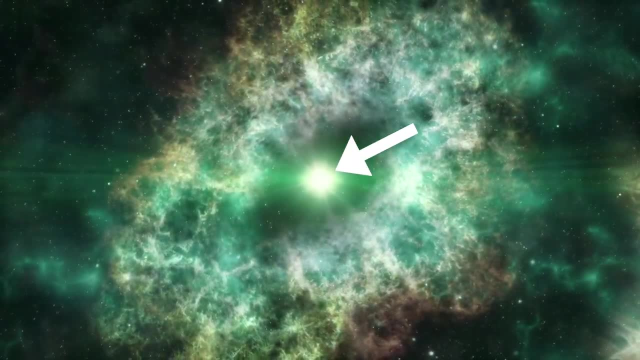 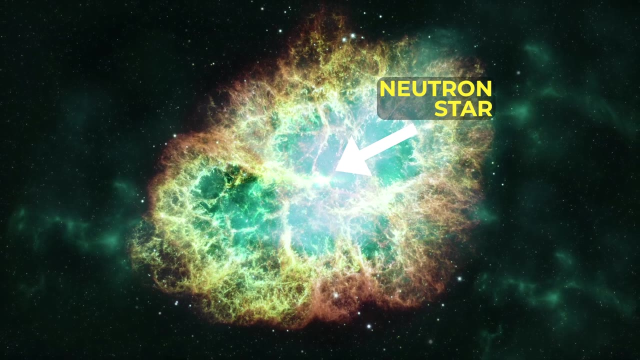 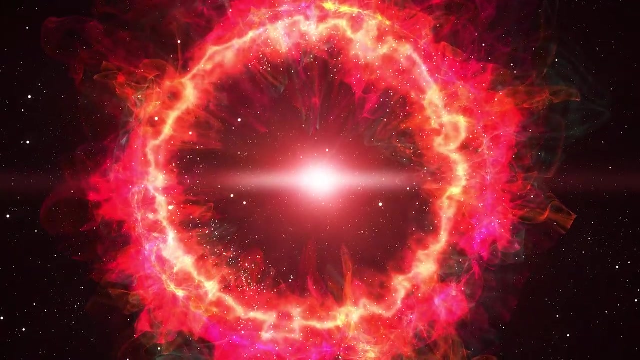 what we call a planetary nebula and the core becomes a neutron star. It can live on for billions of years in this state, slowly cooling down into a black dwarf. We call the cloud a planetary nebula because we used to think that this is how planets formed. 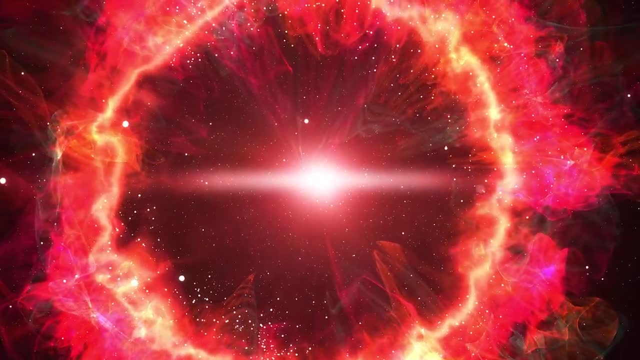 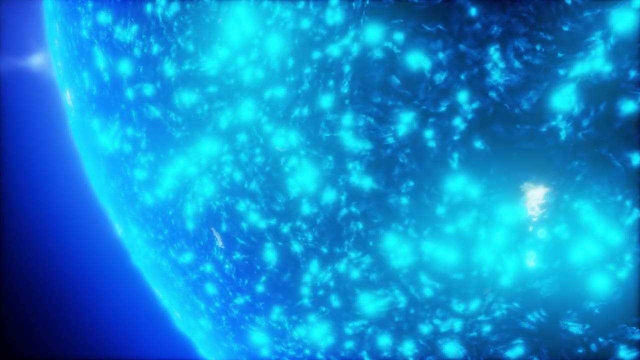 Later this turned out to be wrong, but the name stuck. The core is called a neutron star because all the elements inside of it were compressed so tightly that they fell apart into neutrons. This is one of the densest materials in the universe. 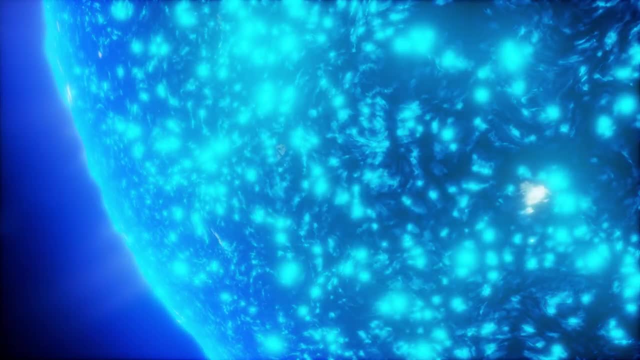 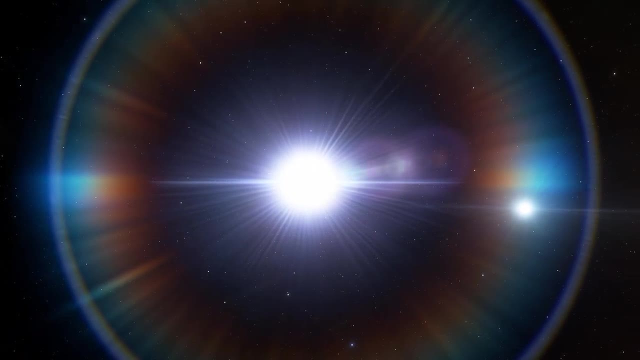 with a teaspoon of it weighing a staggering 4 billion tons. Now, heavier stars are not much different at first, except that they start out shining blue light. These stars live much shorter lives than our sun, with a 60 solar mass star living for. 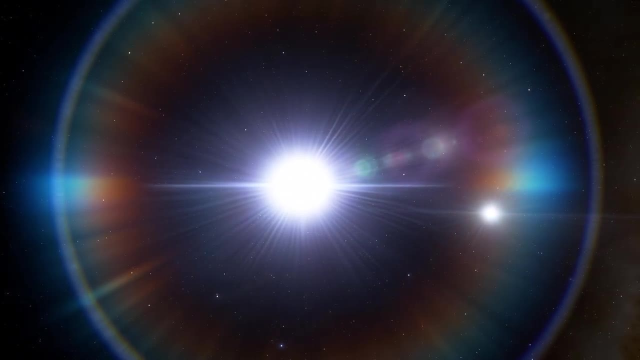 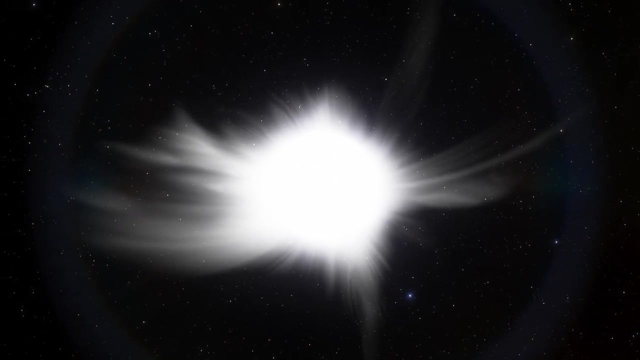 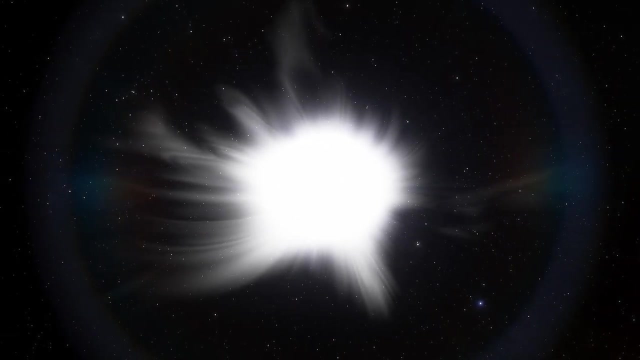 only 3 million years, but burning up to a million times brighter than our sun. Once their time is up, they will become a supernova. At first, they will do the same as the low-mass stars and burn up their hydrogen. Then they expand into a red supergiant and start burning helium. 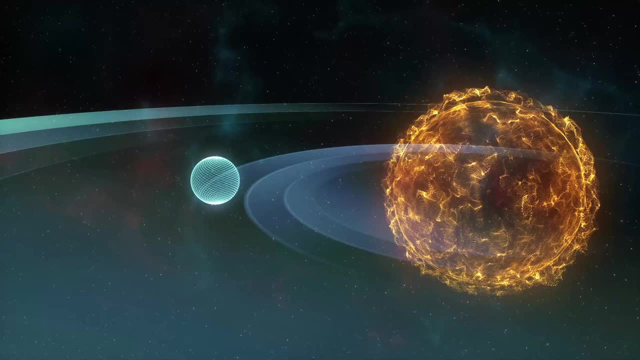 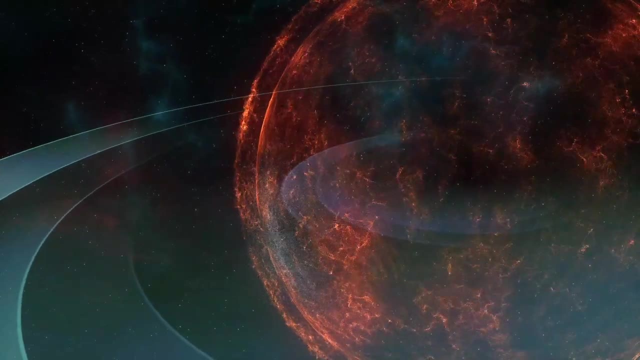 and even some heavier elements. However, the star will run out of fuel at some point and the core will start collapsing, But this time the collapse will not stop as easily and compress the core until something happens that causes the star to collapse.